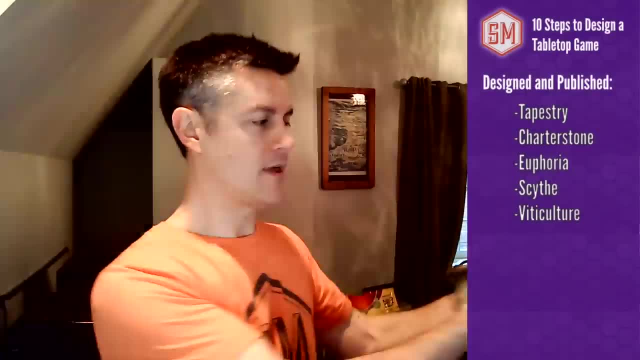 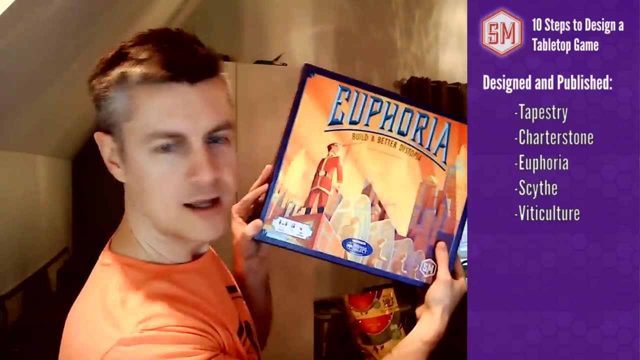 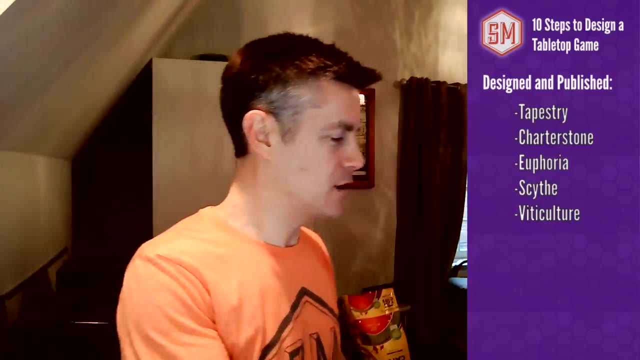 Most recently, there is Tapestry. Before that there was Charterstone, Then there's Euphoria And- sorry, these are all over the place. Here is Scythe, And then Viticulture is here as well. There we go. I'll probably be mentioning some examples from these games in this video. 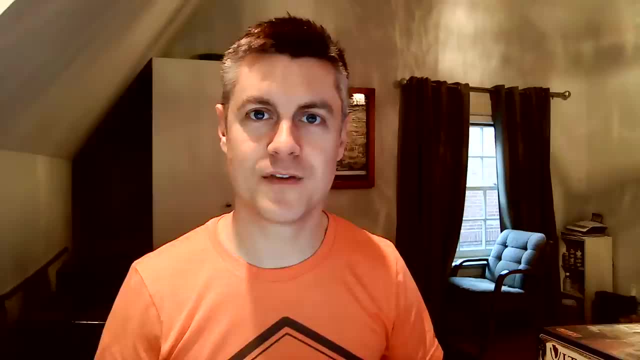 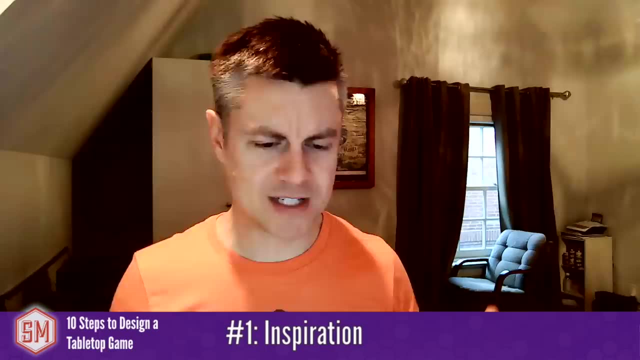 but I am going to try to keep this video to just 10 minutes so that you can figure out the 10 steps to design a board game in just 10 minutes. The first step for me is inspiration, Inspiration, just getting that initial idea Before even I start the brainstorming process. 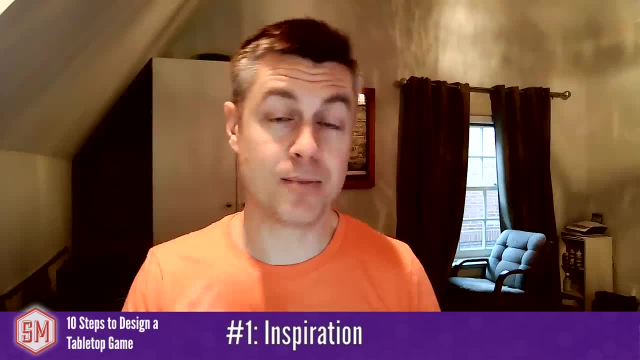 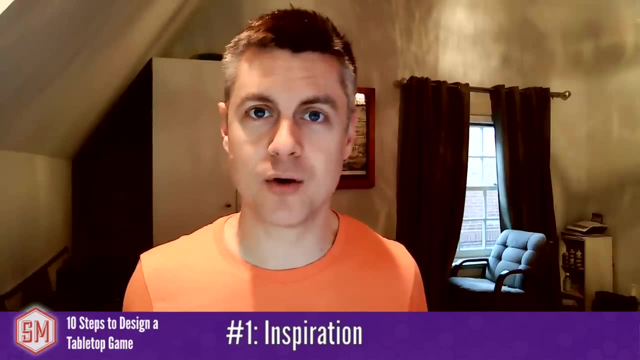 I'm trying to get inspiration. Inspiration- I start by playing a lot of published games. I play games that are like the games that I design. These are medium weight Euro games, but I also play a wide variety of other games because I want to get ideas from a variety of other games and have them improve the games. 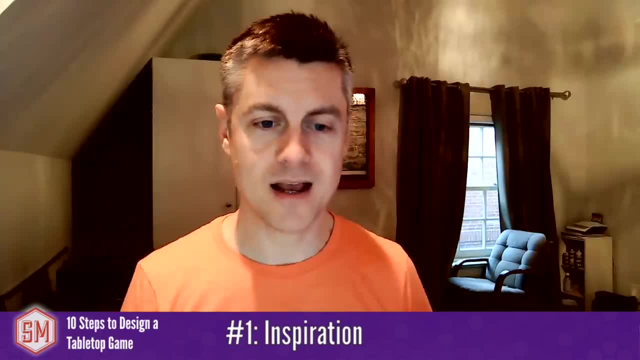 that I'm making And they often give me ideas. I watch a lot of reviews of board games and some videos about video games and digital games, because those give me ideas as well. I read a lot of fiction. I also watch a lot of fiction. 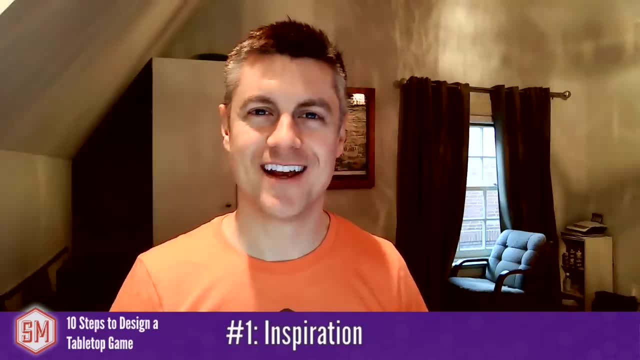 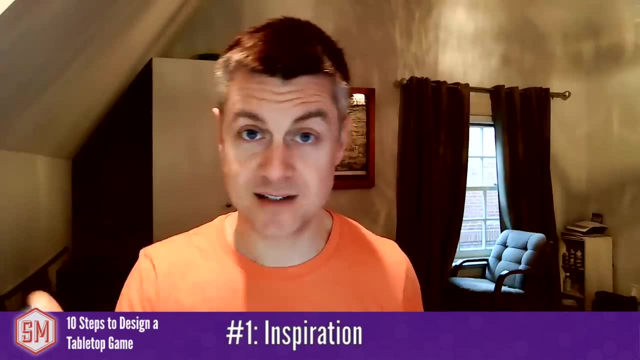 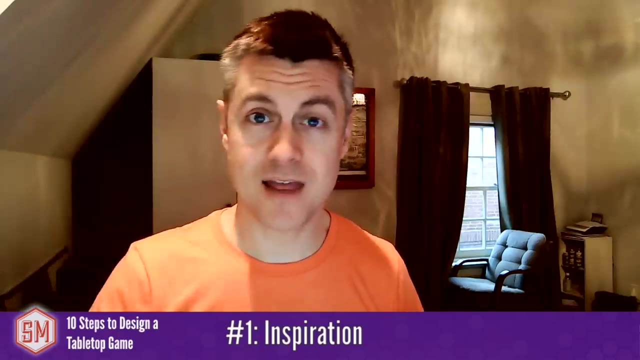 I love movies, I love fictional television shows and especially reading. It gives me ideas for the worlds that I'm trying to build, for games And for all these ideas. before I even get to the brainstorming stage, which is next, I try to track them in Trello. Trello is T-R-E-L-L-O. There's links for that and anything that I'll. 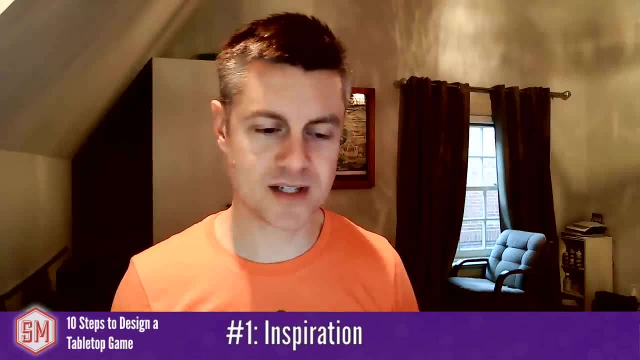 mention in this video in the description of the video. Trello is a nice place for me to jot down a quick idea. It's a list-making app, a list-making web app. So if I have an idea I don't ever forget about it. So I jot it down in Trello and I revisit it And that's. 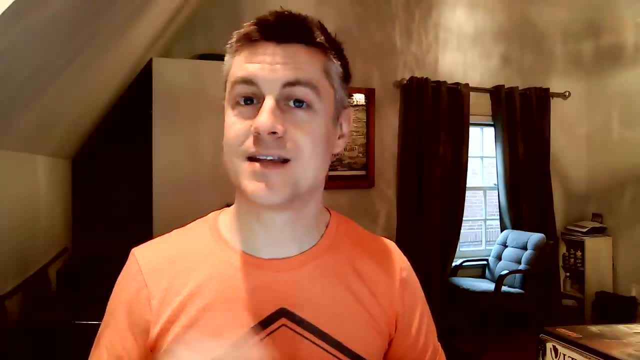 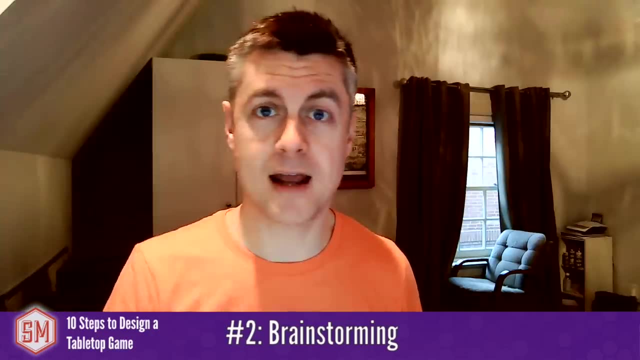 it for this video. Thank you so much for watching. I'll see you next time, Bye-bye. Step 2 is the brainstorming stage. For me, this involves turning off my computer and, either at my desk or at a coffee shop, I just write down ideas, Pencil and paper. I either 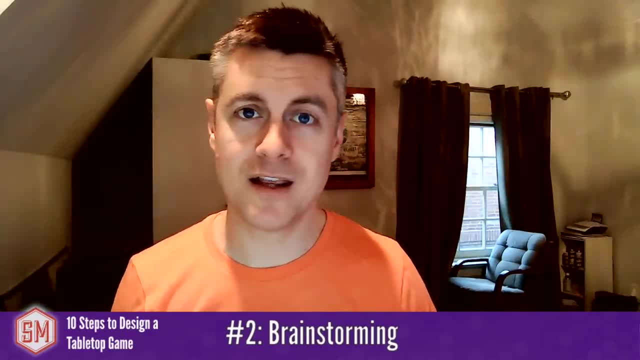 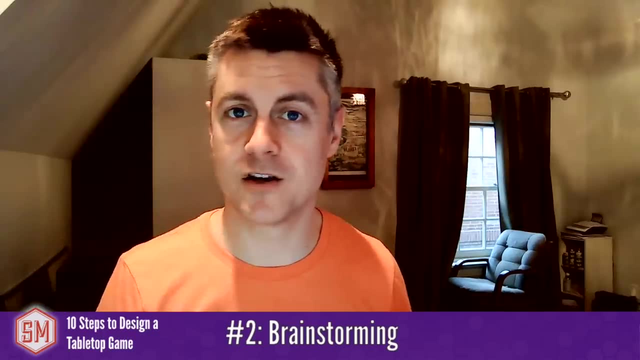 start with a theme or a mechanism. It doesn't really matter, because as soon as I write down a theme, I'm thinking of mechanisms that go along with that theme, And then I'm thinking of parts of the theme that go with that mechanism, and so on. For me it's pencil and paper. 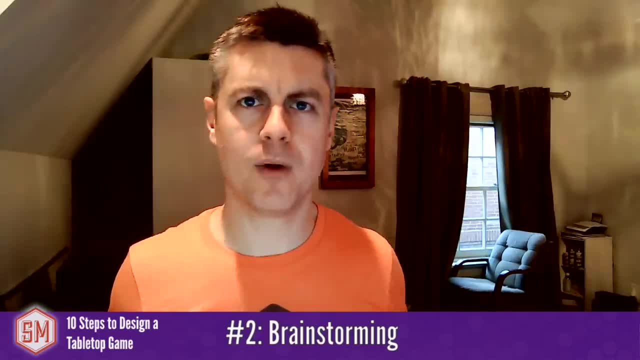 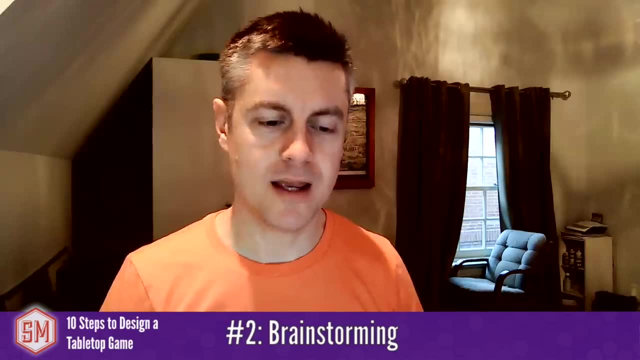 Sometimes it takes a week To brainstorm a game. sometimes it takes several months when I'm just kind of going back and forth between that and other projects. I don't think there's any limit to how long you can brainstorm. It is important for, eventually, for you to move on to the next step. I think 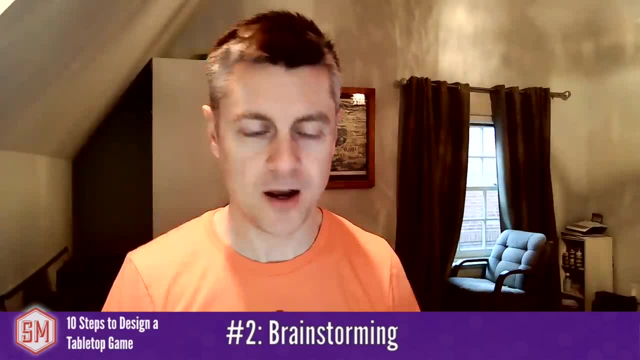 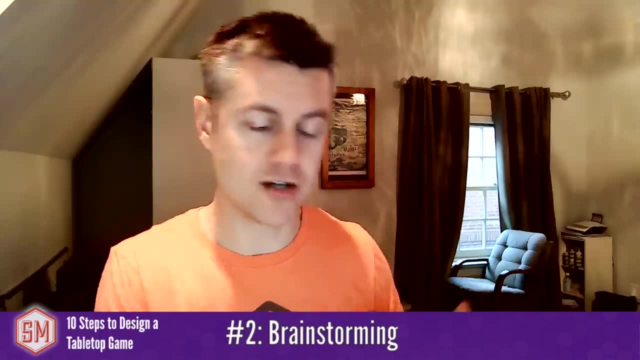 But for me, I really enjoy the brainstorming process, So I spend some time doing it. I also try to have more than one game in the works at any given time, So if I'm really excited about brainstorming one game or working on one game, I can jump around between that. 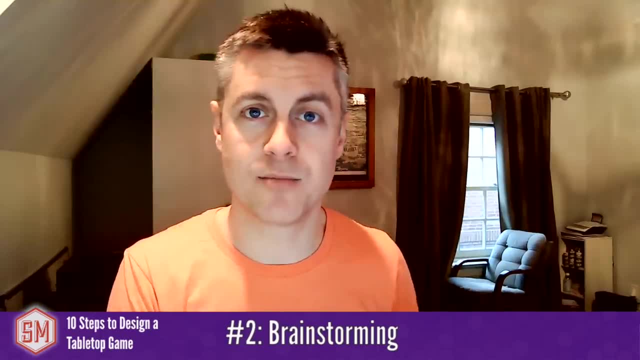 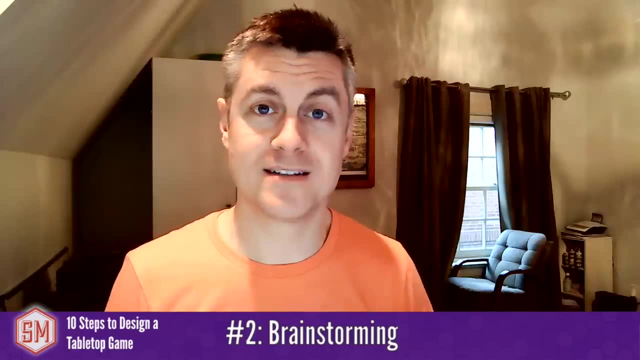 and another game that might end up being at a very different stage in the design process as the other game. Most importantly, at this point in time, when you're brainstorming, you might have some really cool ideas and that's great, but they are still just worthless at this point. 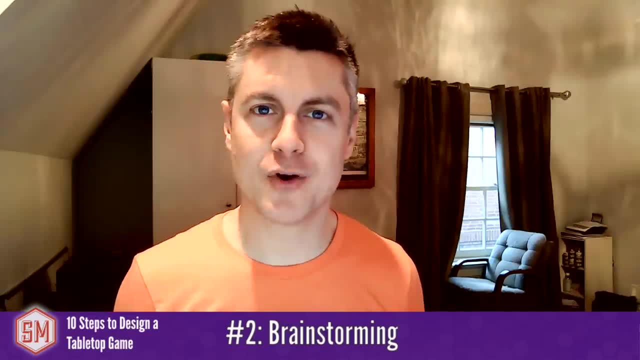 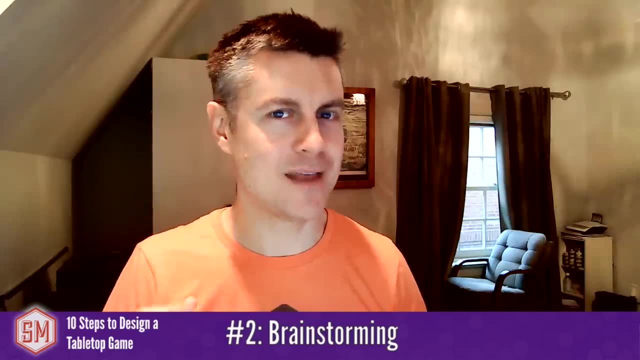 What matters is execution. So I'd recommend not keeping your ideas too close to your chest and actually just sharing them with people a little bit online and share them with friends, because they might say, hey, that game, that exact game you just mentioned, already exists. 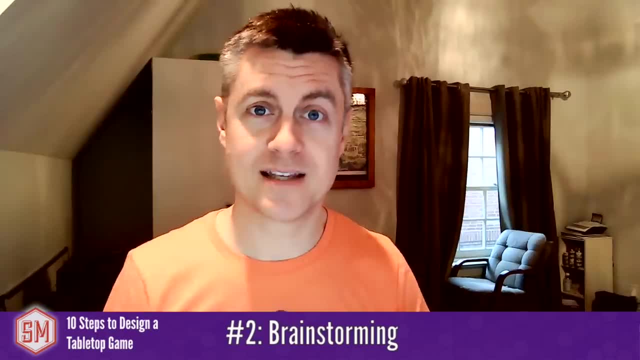 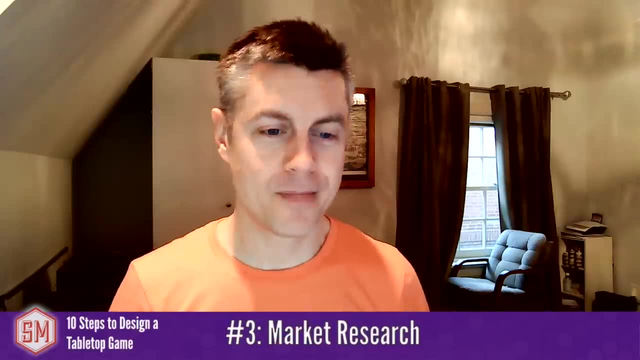 Or they might say that doesn't exist. That sounds really exciting Work on that. I'm excited about that. That's step two. I'm already a little behind pace here. Step three is market research. See what people like or dislike about the genre of game that. 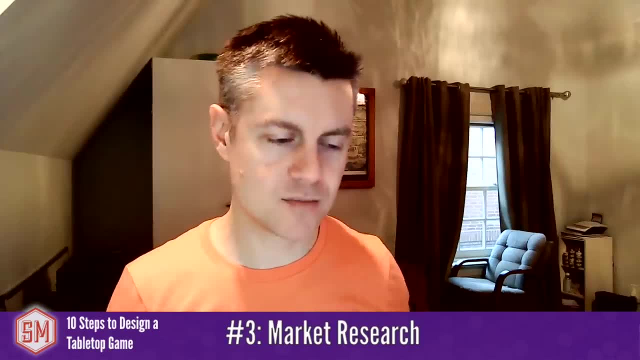 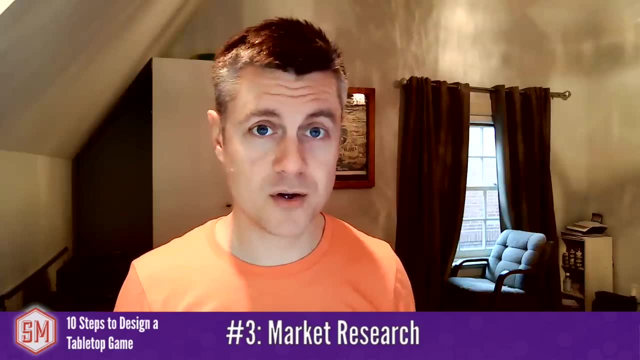 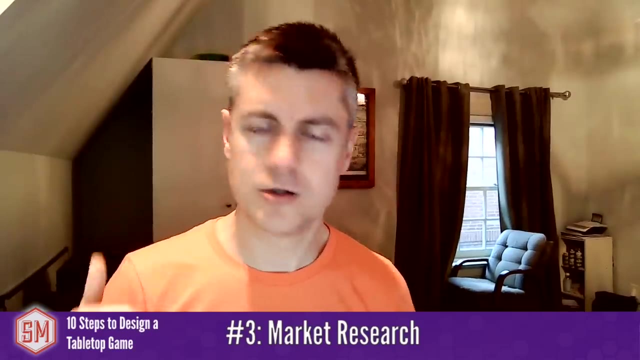 you're designing, whether it's the mechanism, the genre of mechanisms or the theme itself. This is where you can both watch review videos about games, but you can also watch or learn from other resources. I mentioned some below in the comments. There's a podcast called 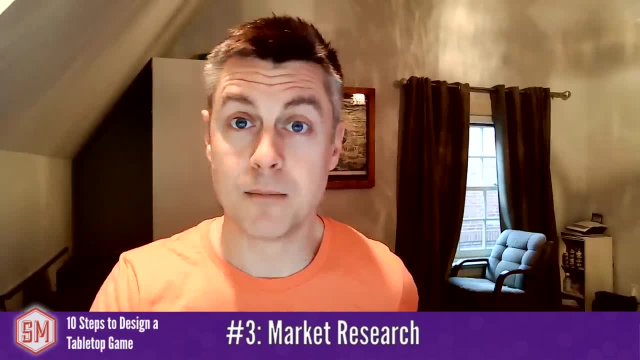 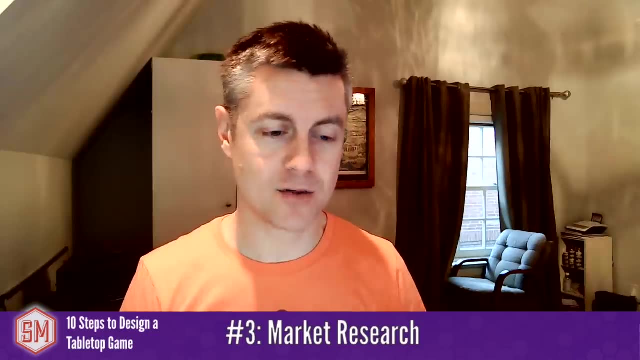 Ludology. There's Board Game Geek. Board Game Geek is an amazing resource That's a big community of gamers, And also more recently, there's one called Board Game Atlas. These are places where you can go to discuss games and game design. There's the Board Game Design. 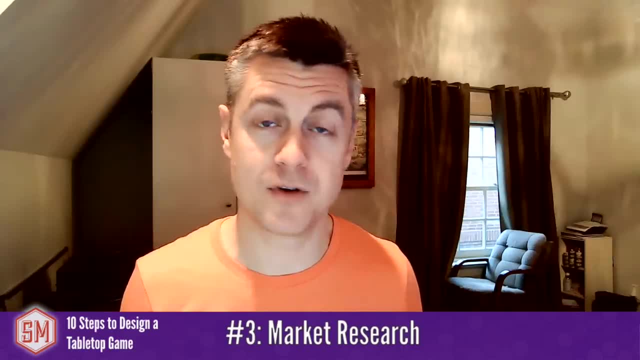 Lab. That's a wonderful podcast about game design. If you're designing a cooperative game, there's the One Stop Co-op Shop. There's also Game Maker's Toolkit that focuses on video games, And there's also my YouTube channel. My YouTube channel is specifically about my 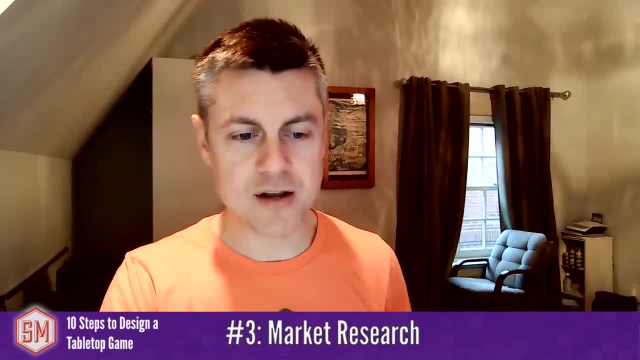 favorite mechanism in a variety of games. And last I'd mentioned, there's a site called Cardboard Edison. It's a great website. It's a great place to learn more about game design. It's a great place to learn more about game. 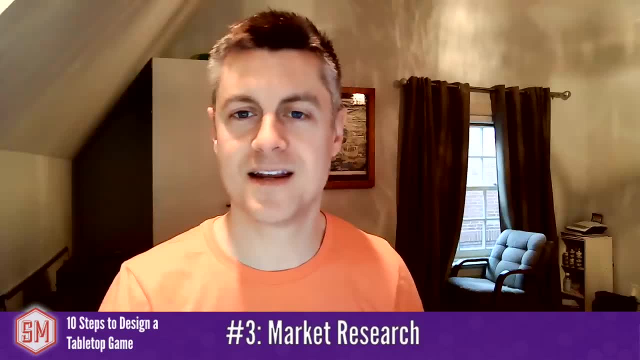 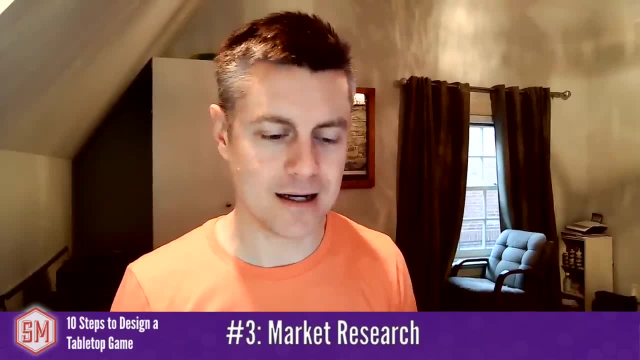 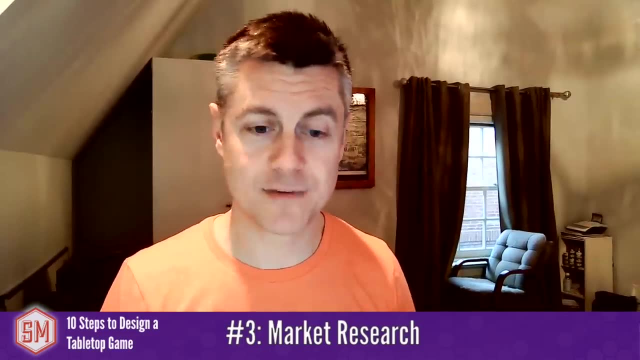 a lot of different game design resources. So this is market research: See what people like or dislike about all these different mechanisms, all these different themes. Look out there to see what has been done, what hasn't been done, And really be active in. 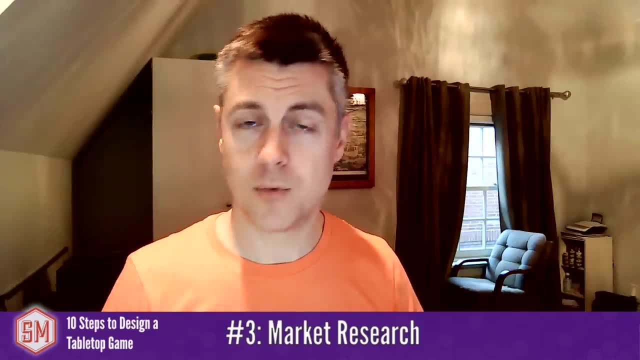 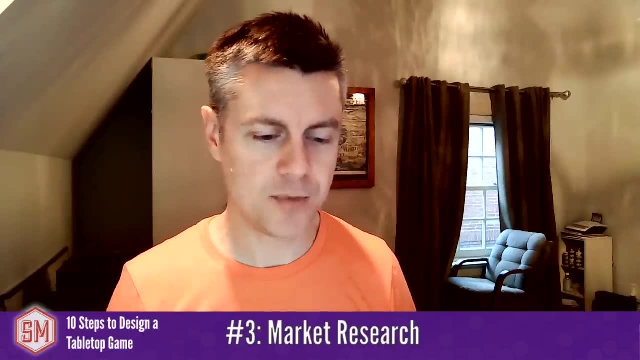 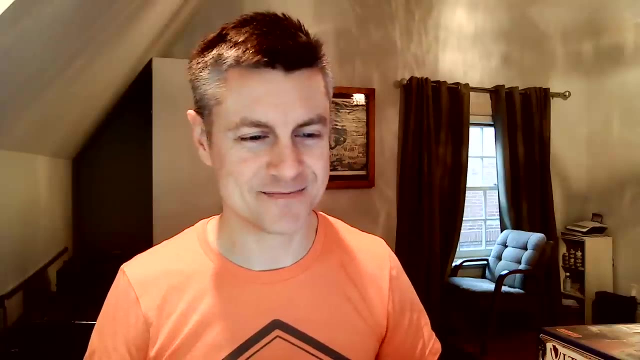 some community, whether it's Board Game, Geek, Facebook. There are game design channels and groups on Facebook or on Board Game Atlas. Any of them can help you figure out what people are actually excited about, what they dislike and don't like, or like and dislike. 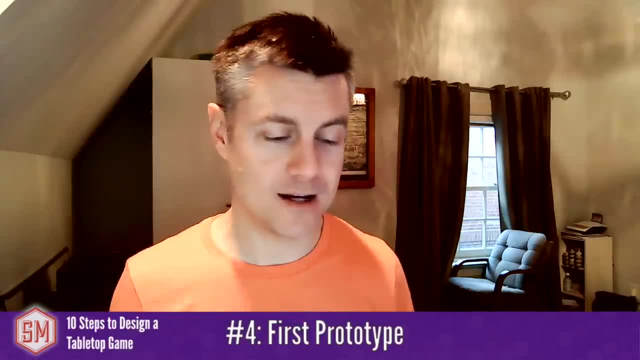 Number four is start making the prototype. You don't want to wait too long to make this first prototype because, however it's playing out in your head, it's going to be very different than once you get it to the table with actual human players For actually creating the prototype. 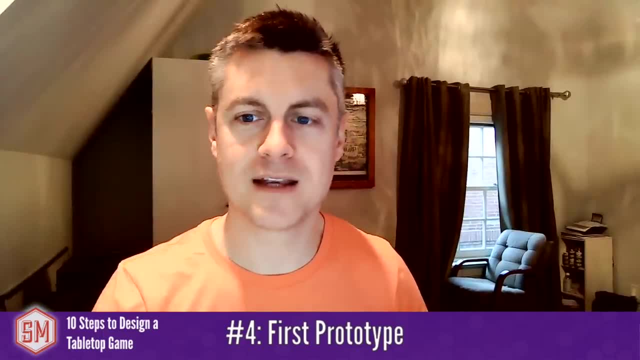 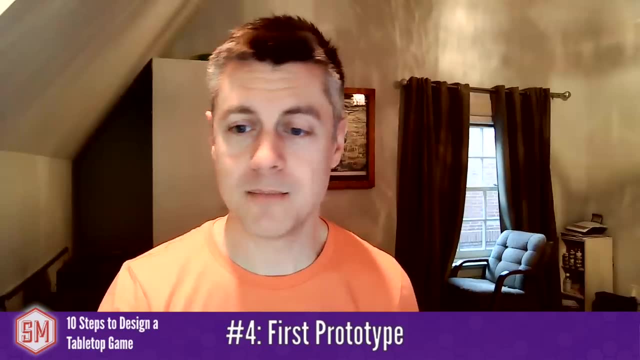 there are a variety of different ways you can do it. It depends on, probably, the weight of the game. If it's a game that only uses 10 cards, you could draw it down on 10 pieces of paper right now and make it, But if it's a more elaborate game, you might use a program like InDesign. 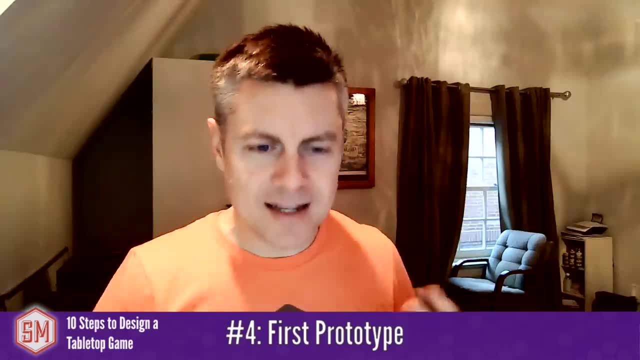 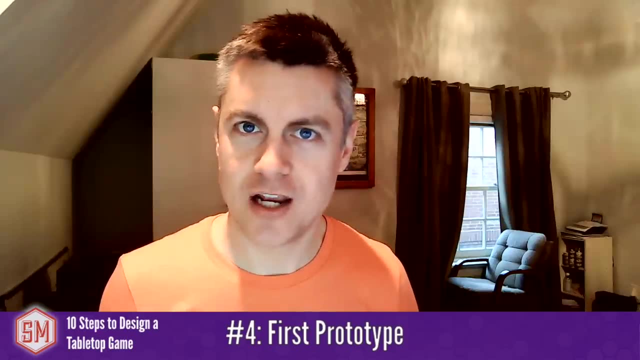 which is what I use When I'm in InDesign. I'm trying to think about the user experience and layout. I know those things are going to change as we actually get to the table, but I don't want those things to get in the way of the first playtest. So I am trying to put myself in the shoes of 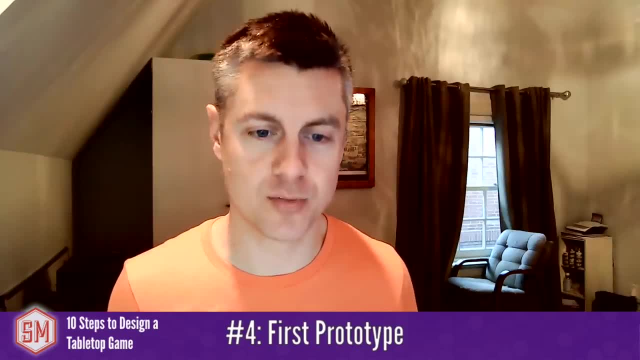 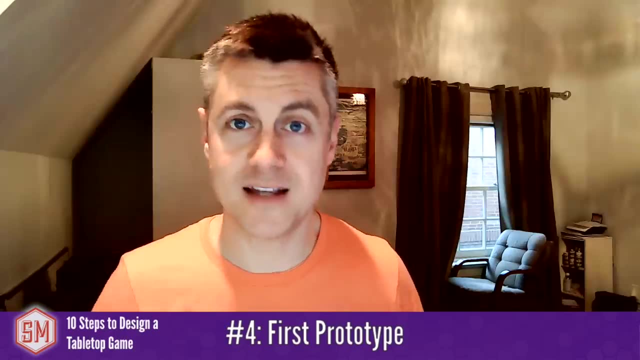 the players of the playtesters. as I'm even designing that initial prototype, I am also thinking about things like: eventually, if this game works out, will my blind playtesters, who just get digital versions of the files? are they going to be able to even make this? 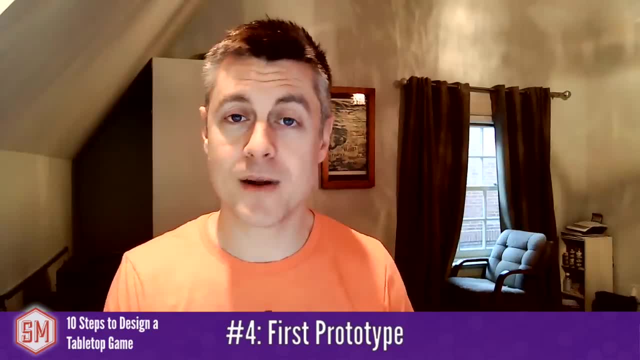 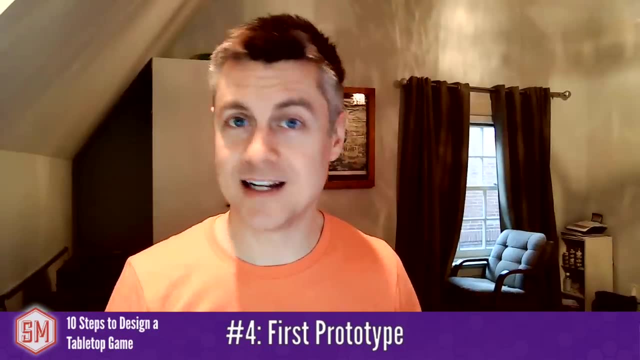 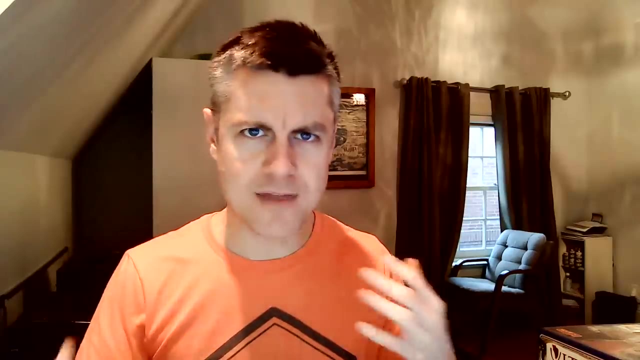 Will they be able to make this prototype? Also, I'd recommend a resource called gameiconsnet. Again, link is below. It's game-iconsnet. That's a great place to get icons that you can use for your prototype. Number five is, as you have that prototype ready, as you're about to move on to internal. 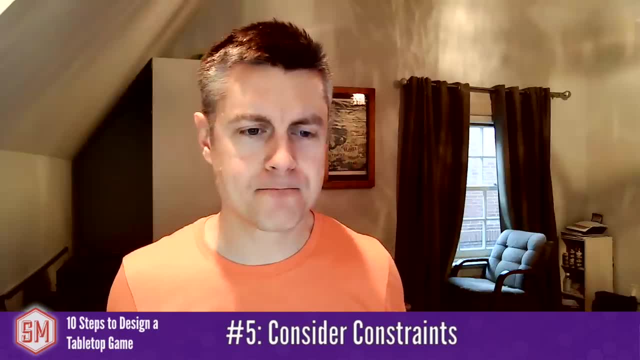 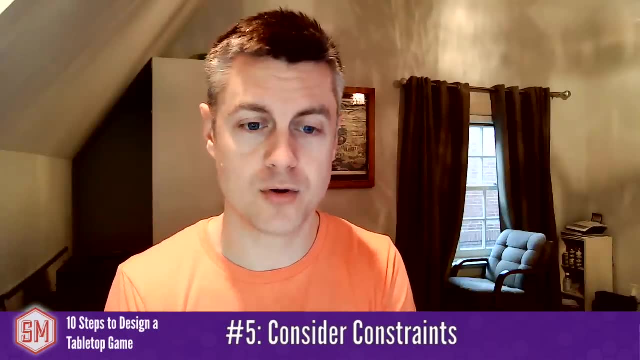 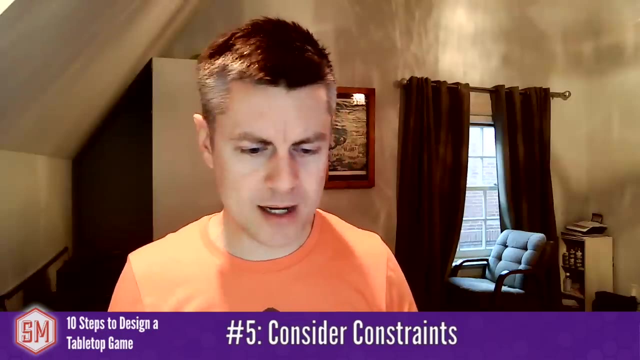 playtesting. consider constraints. Constraints like initial costs, like what I said about. will playtesters even be able to construct this prototype in the first place? And it all comes down to who are you making this for. So, if you're making a game for an audience that is willing to pay $150, components aren't. 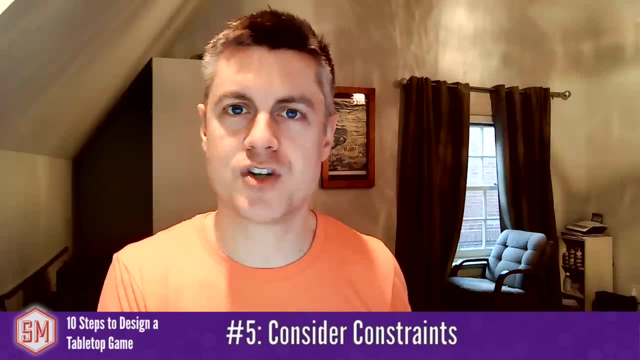 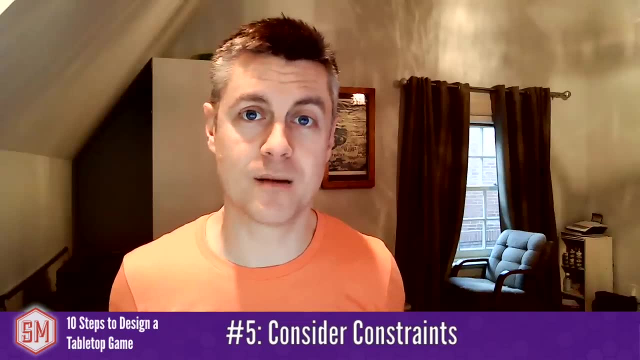 going to really limit you, But if you're trying to make this a game that might end up on the shelves of Target, then it's got to be around $30 or $40 at most. So even from the early stages of design, you might need to start thinking about components. 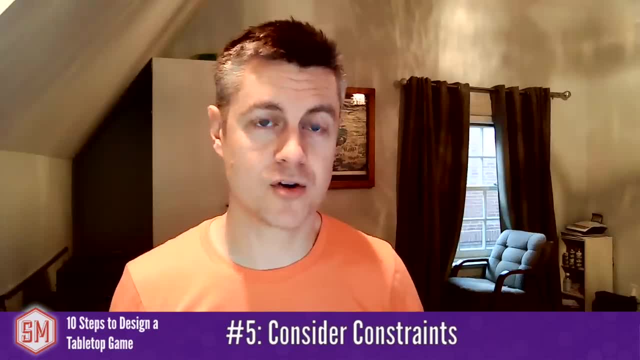 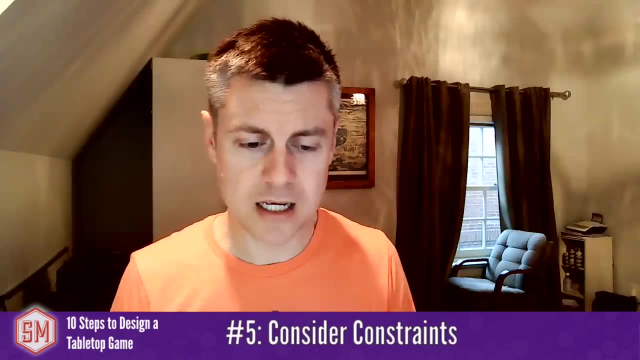 One thing that I do during this process, because I'm both a designer and a publisher, is that I might send Panda. I use a company called Panda Game Manufacturing. I might send them the early ideas that I have for the components, just to get a rough idea for how much they're. 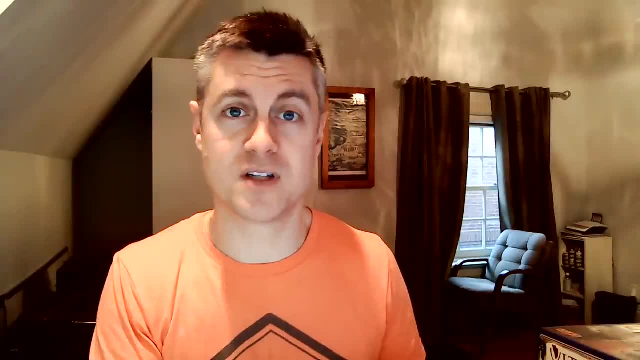 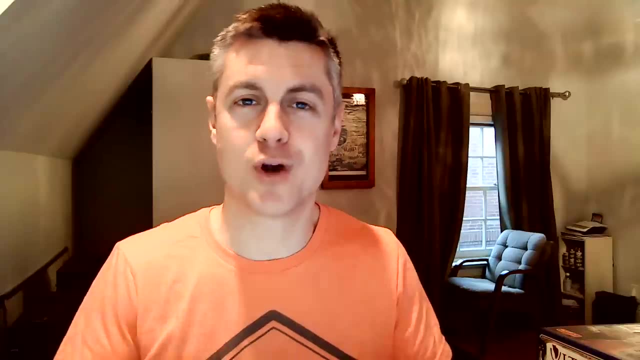 going to cost to make. so I can know, hey, it's actually possible for us to make this game and make it on a reasonable budget and sell it at a reasonable price, or not? Or maybe I need to cut this giant, awesome metal component. 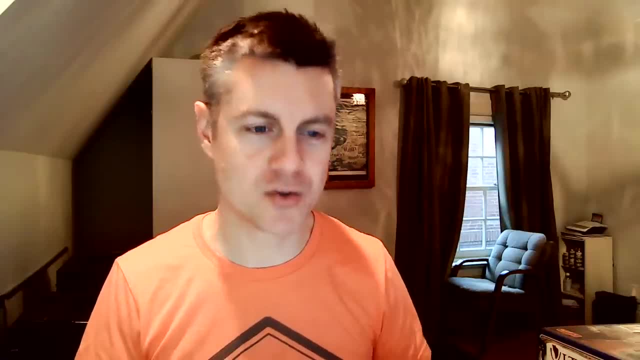 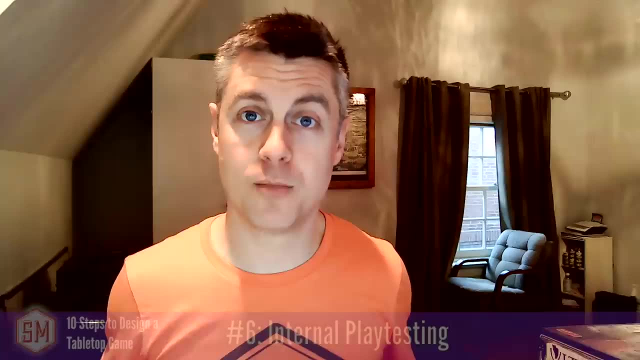 That I thought would work, but it's going to cost way too much, So it's really nice to have those constraints from early on. Once I have that, once I have that prototype, that audience in mind, I start internal playtesting. 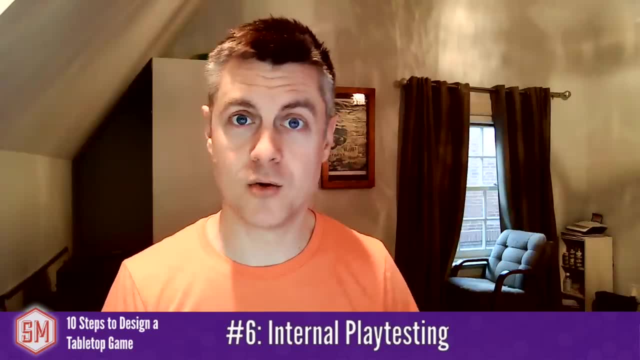 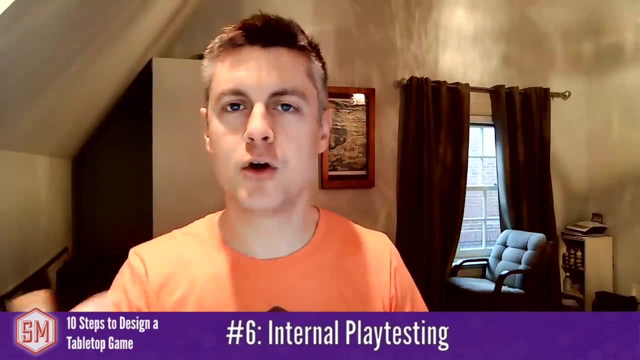 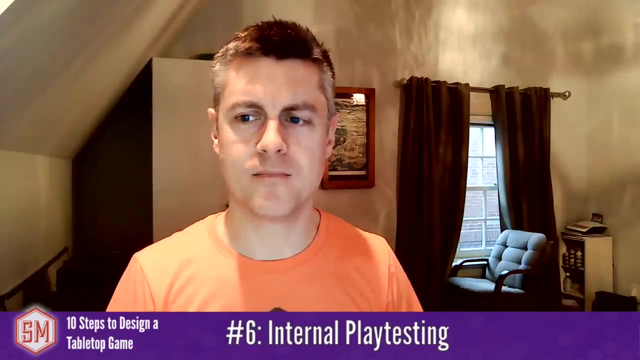 Internal playtesting for us. I have a company and so I gather with my coworkers and we playtest the game. That's internal playtesting For you. if you don't have a company, that might mean that you're playtesting the game with a few, maybe family, with friends, Really. 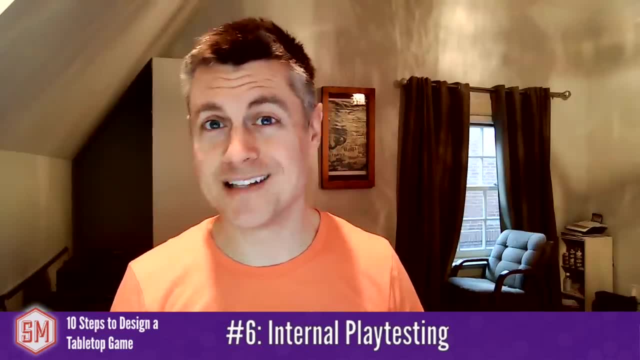 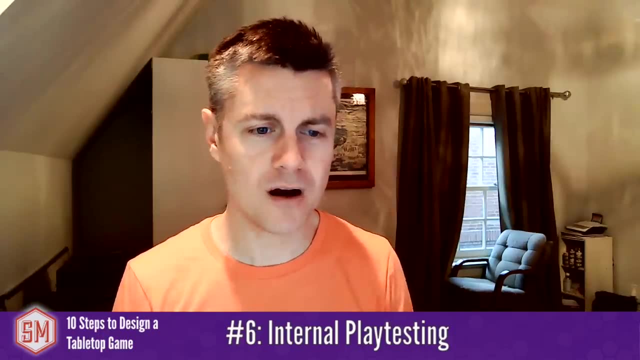 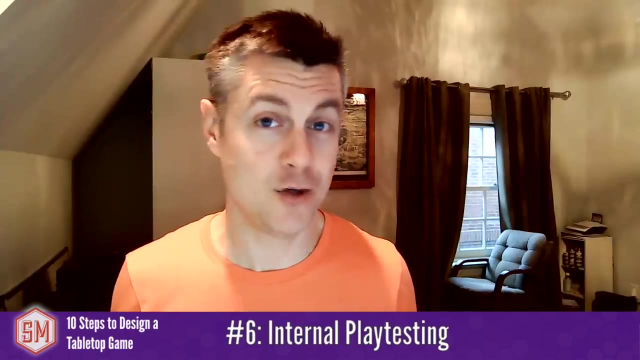 really like isolated, local playtesting, The types of people that you don't mind sitting down with and that they might even have a bad time with it because they're probably not going to really enjoy that first playtest. all that much Internal playtesting for me, I mean. I've never had a game be awesome in the first playtest. 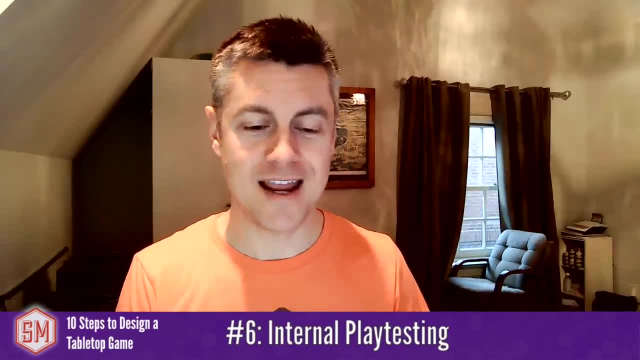 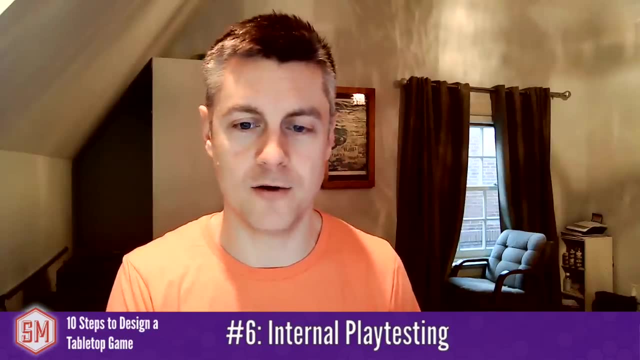 Usually it sucks And that's okay. I'd go into it knowing that it's not going to work and that I'm going to have to change things- some of them on the fly, some of them after the playtest- And then I do it again. I continue to playtest it internally for a while. I'm 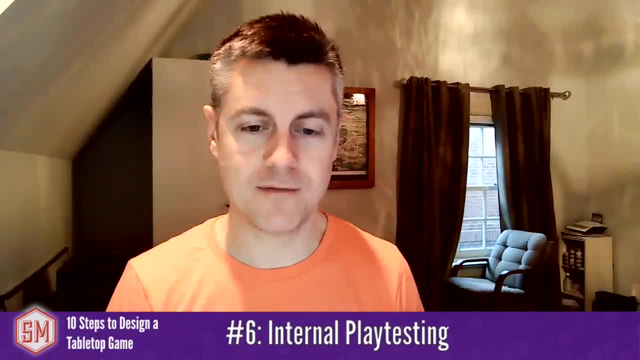 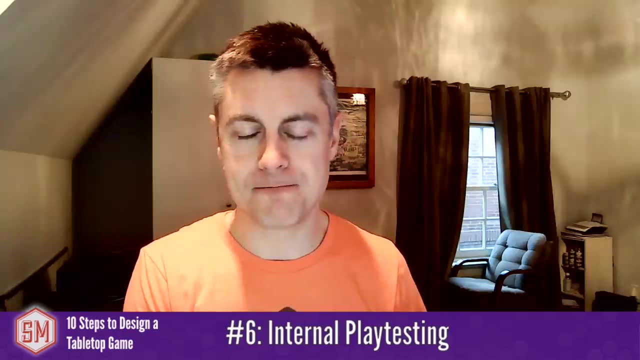 also, I go into these internal playtests knowing that I may not have everything figured out, I may not know how the game ends, and I may be playtesting just to see, hey, what makes sense for when the game ends. But one thing I am paying attention to from the very beginning: 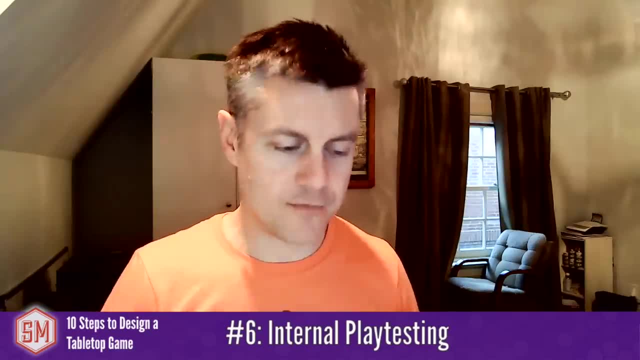 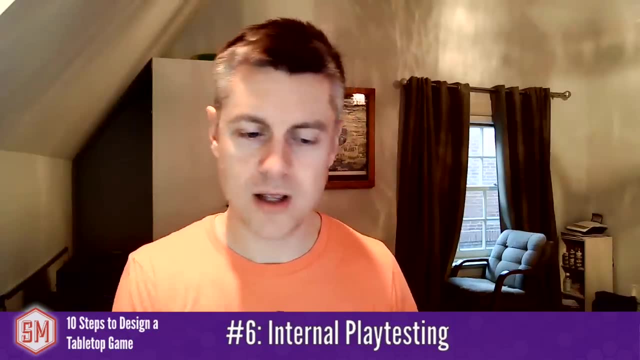 is the flow of the game? How are players, how is the game flowing from one turn to the next, Even from those early stages when a ton of the mechanisms may later change? I want to know if it's a smooth flow or if it's a real awkward flow. That's the thing I really. 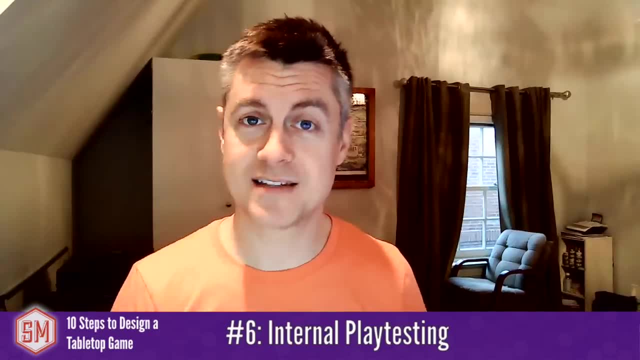 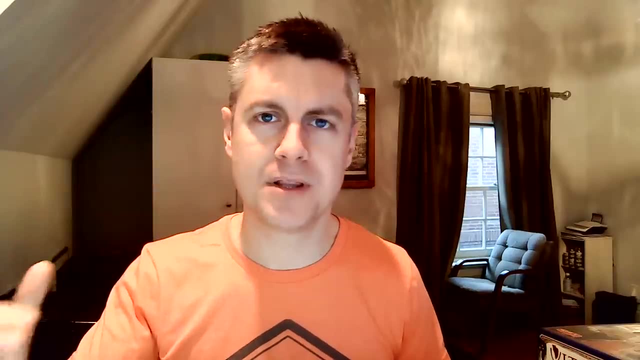 try to pay attention to. At this point, and after several of the next steps, I might stop. I might say this game is just not going to work. I can tell it's not going to work. What I thought in my head. it played out completely differently than it does in real life and I might just stop. 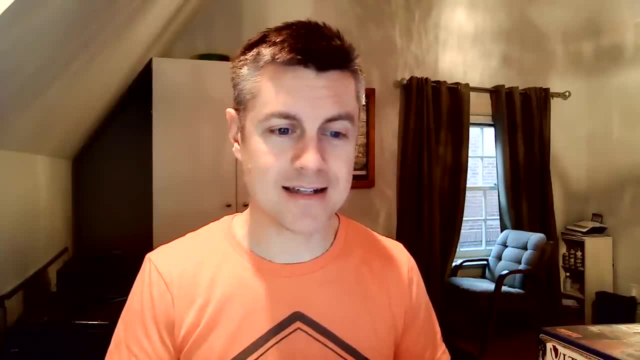 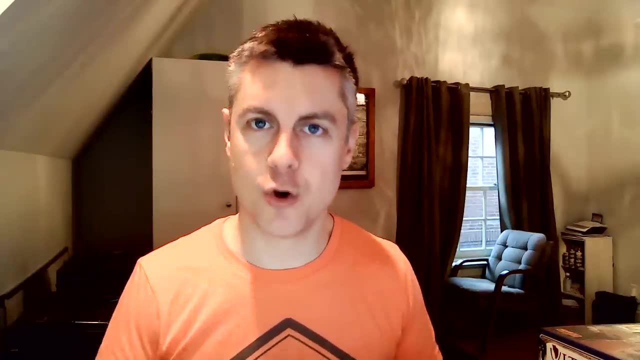 But if I don't, if I think the game has potential, then I continue. And I continue that internal playtesting until the game is halfway decent, until it's functional at least, And then I expand it to local playtesting. This is kind of a broader reach out to friends to meet. 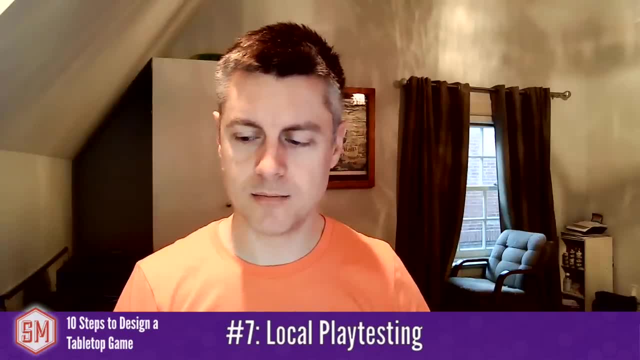 up groups in the area. Events like Unpub and Protospiel and the Stonemaier Games Design Day, where people come together to playtest games locally, all locally, where I'm there at the table actually teaching the game and playing it with other people. 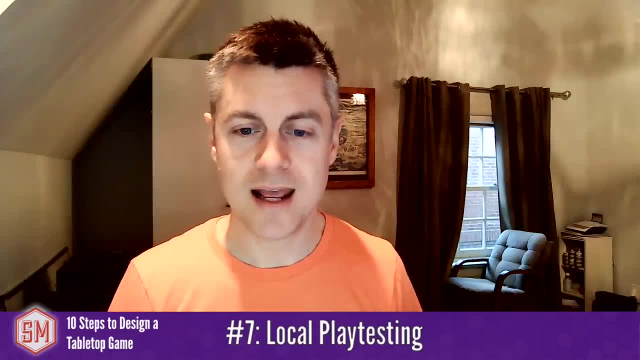 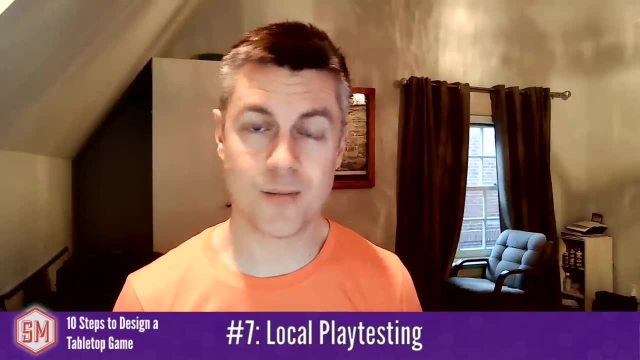 And at that point in time I'm often paying attention to what's fun and frustrating and just to see what players are. I'm also watching players see how they interact with the game, what's enjoyable for them, what's not fun, And I try to pay attention to myself as I'm teaching the game, to see how many times I 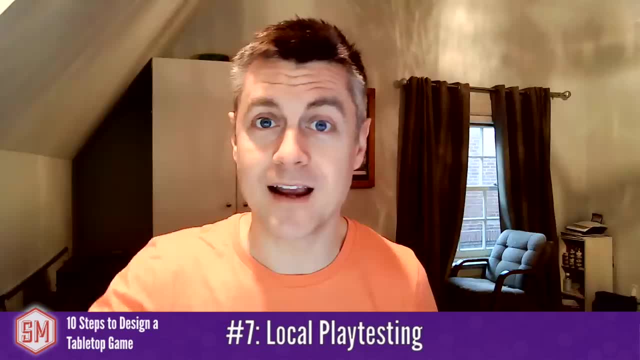 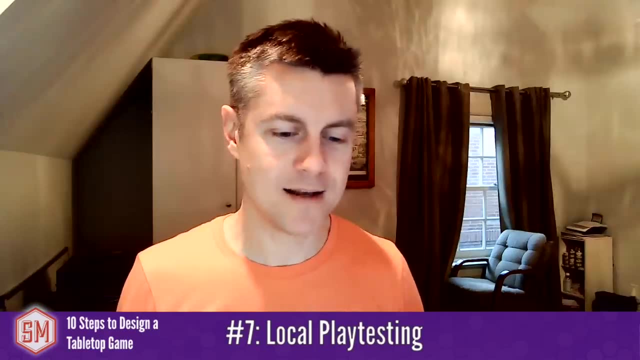 say words like remember, Like remember to do that, remember that this icon means this, Because whenever I say that word, it means that the game's interface isn't doing its job. It's not communicating all the things that players need to know, because I'm constantly. 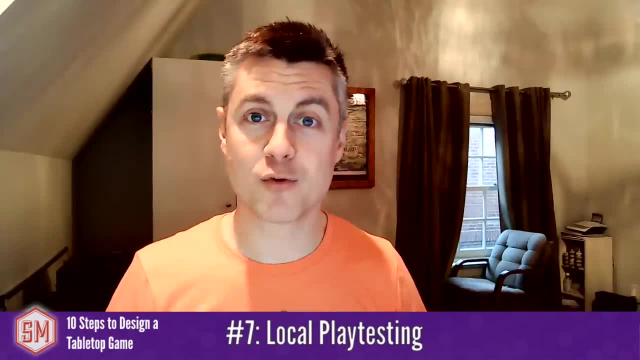 having to tell them to remember this thing. So if I am saying that word remember, it means that I need to improve the game's interface so that I don't have to say that word Because I'm not going to be there in real life when people are playing the published. 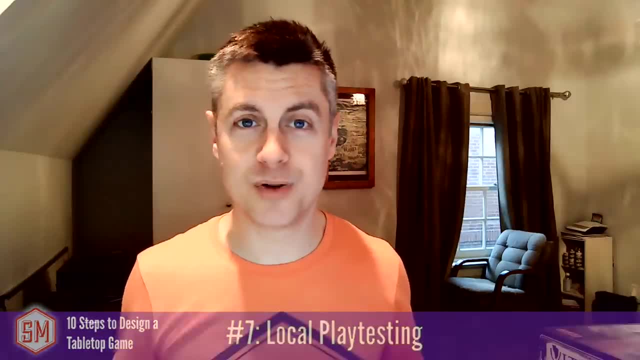 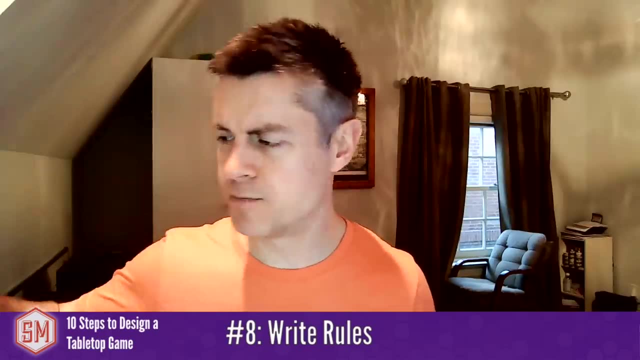 version of the game to help them remember After local playtesting. this is usually when I write the writing. I sit down, I use past rulebooks, I use rulebooks from other games and I sit down and I try to write the rules in the best way possible. 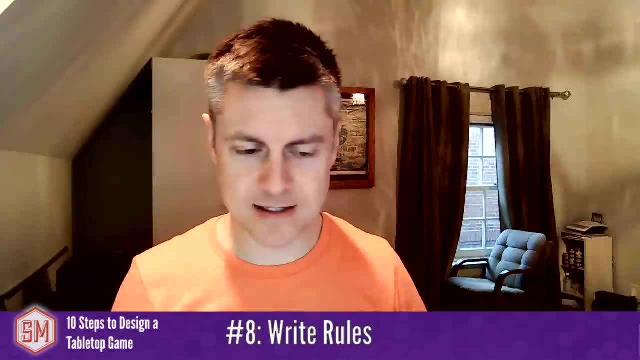 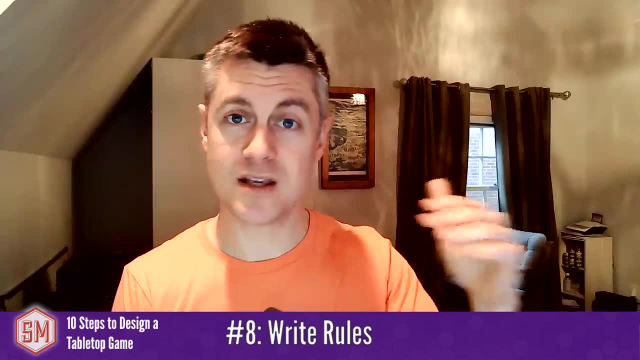 There are many different ways to write a rulebook. I try to use plenty of visual examples. I think they really help. I try to use numbered lists- do this, do this, do this- and I try to break it down in different 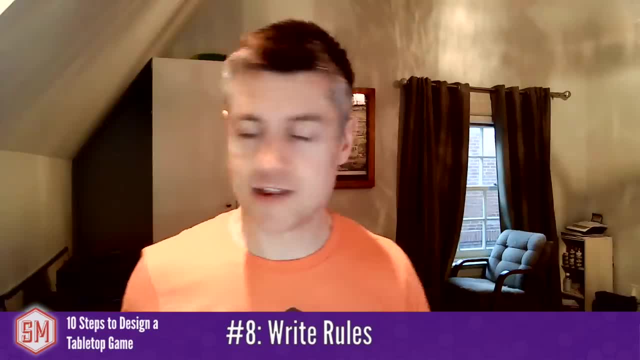 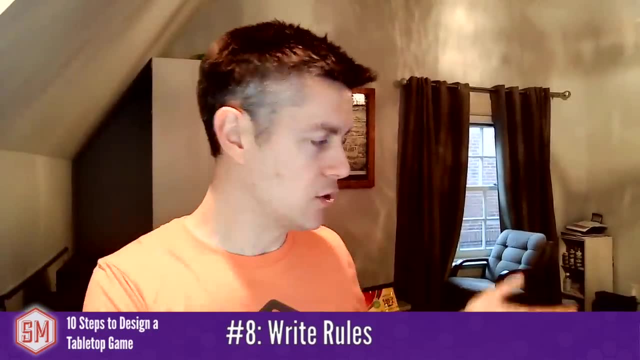 sections. There are many different ways, but if you like the way I mean, you can look at our games. you can look at Tapestry- I really focus on the rulebook for Tapestry. I try to keep it as streamlined as possible- and you can look at our other rulebooks as. 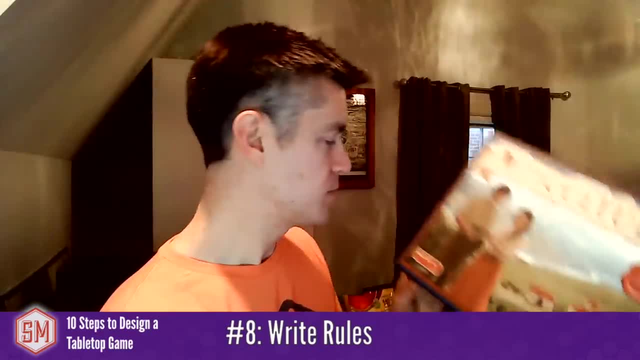 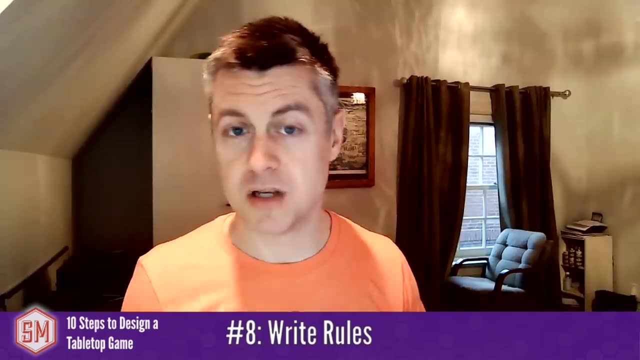 well if you'd like. There's a Viticulture has a slightly longer rulebook, but it works pretty well. Scythe's rulebook is probably the longest. Scythe's rulebook is around 32 pages, but it has plenty of space to give examples lots. 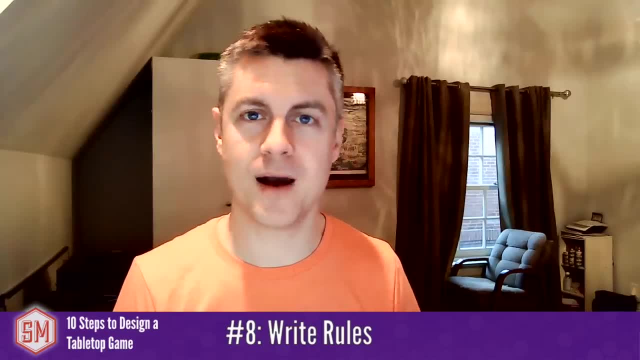 of visuals in the Scythe rulebook. One thing to keep in mind here, actually two things. One is: if you are needing players to remember, say what icons mean and you don't want to say that word, remember over and over again. 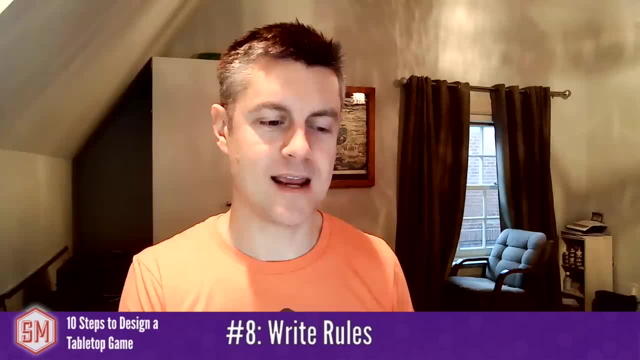 As you write the rulebook. this can be a good time to create a reference card, so that playtesters have a reference card that they can use- one for each player- to remember what those icons mean. And also this can also be a time where you consider outside development. 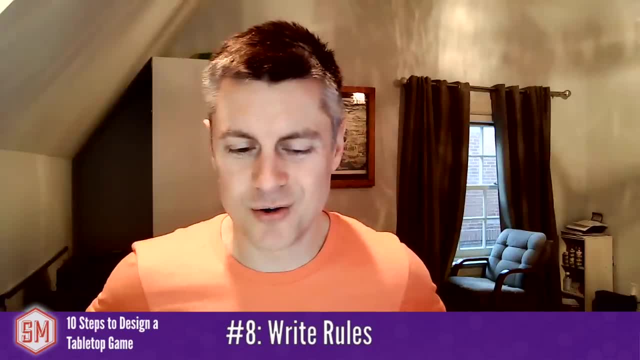 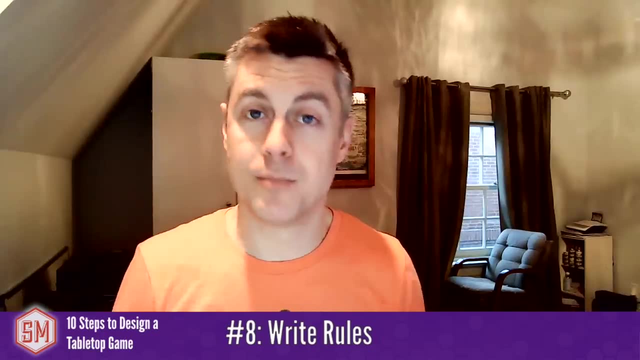 Maybe you think the game isn't quite ready for blind playtesting, and so this can be a time where you maybe hire a developer to take the game to the next level before it's ready for blind playtesting, And the developer may even blind playtest it themselves. 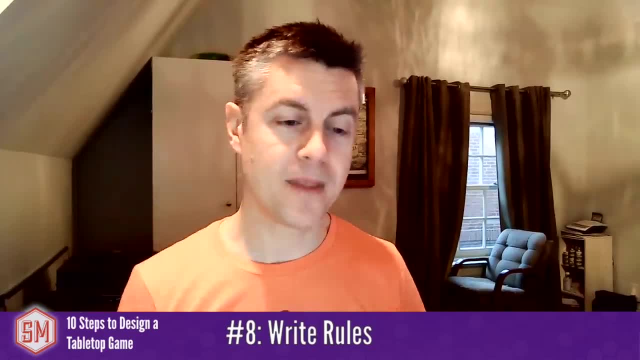 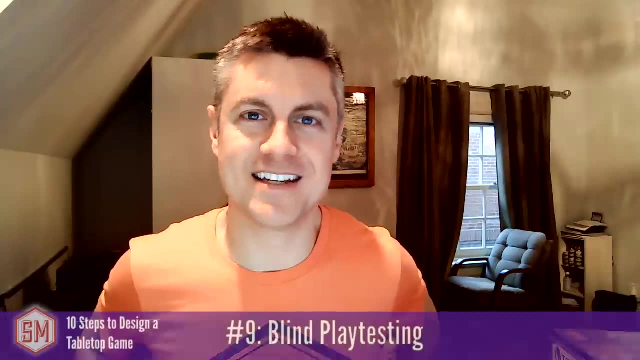 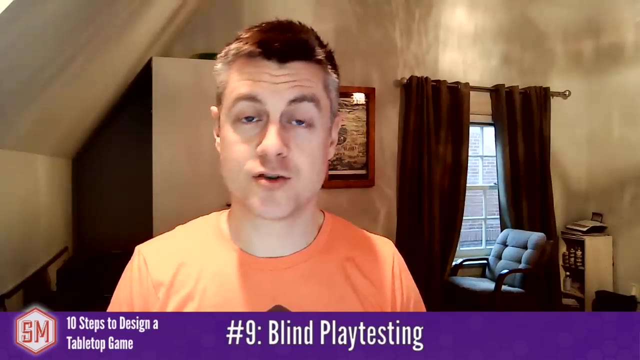 The developer is someone who takes a game that has already been designed and they make it even more fun, even more balanced, even more intuitive. Step nine is the blind playtesting stage. The way I do it at Stonemaier Games is that I send digital files to groups of playtesters. 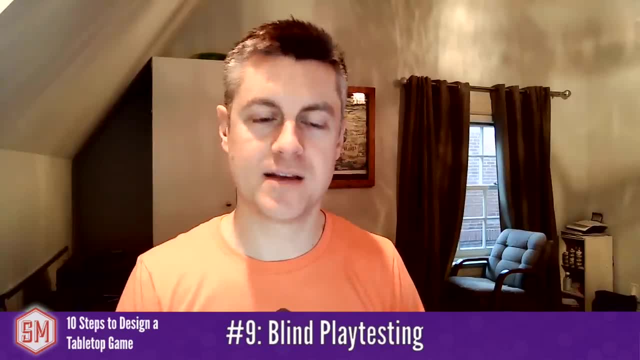 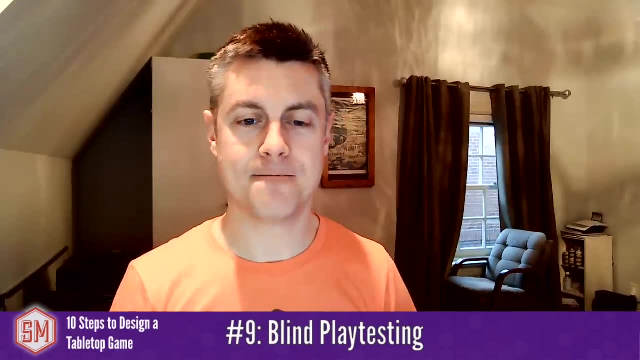 around the world, or lead playtesters around the world that have groups that are ready to play the game. Those lead playtesters print the games at home. They play it. We pay them for their time, And these are people that I vet. 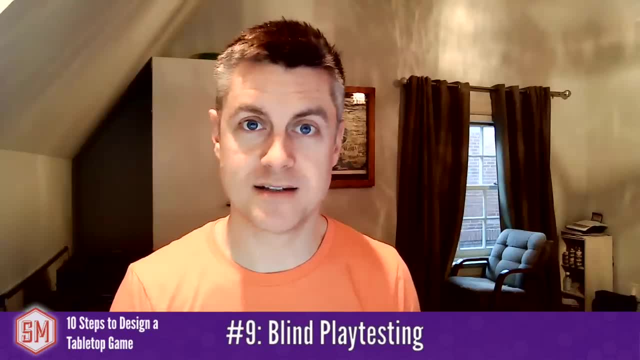 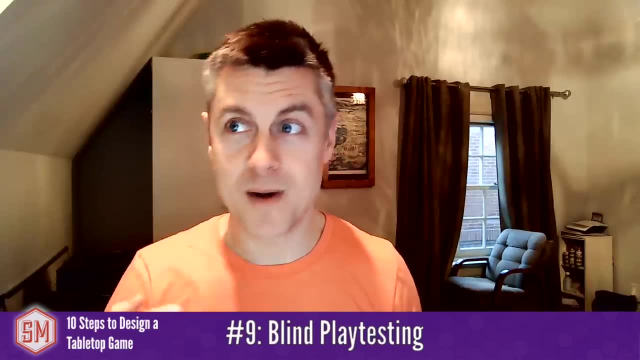 These are people that I've decided are really really good at playtesting. They're good at getting playtesters to do different things, to try different things, and they're good at responding in written form. I prefer written form to provide constructive feedback. 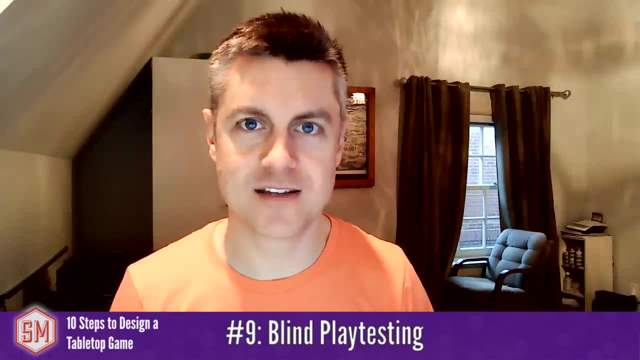 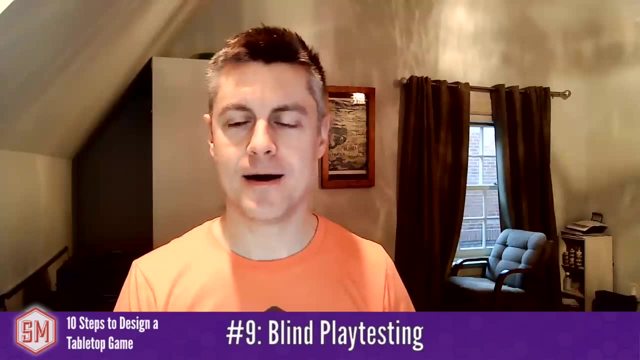 They don't just say you need to fix this or this was bad. They say this is what happened. this specific scenario happened and it was frustrating because of this, And I take that and I can decide what's best to do next. 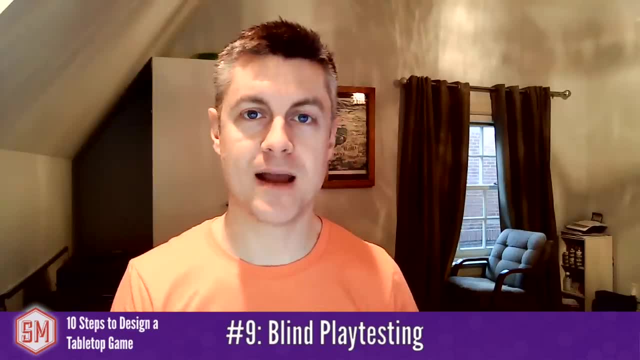 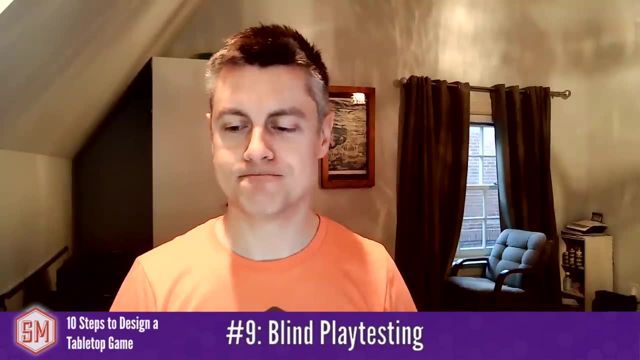 That sort of example-driven, reason-driven feedback is really, really helpful from blind playtesters. If you are looking for blind playtesters, that can be a bit of a challenge, But I would recommend that just start sharing your work with other people. 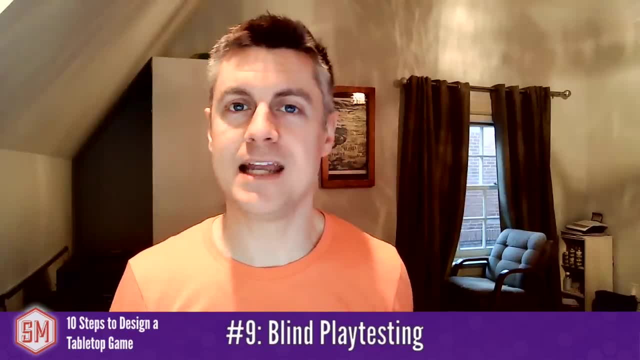 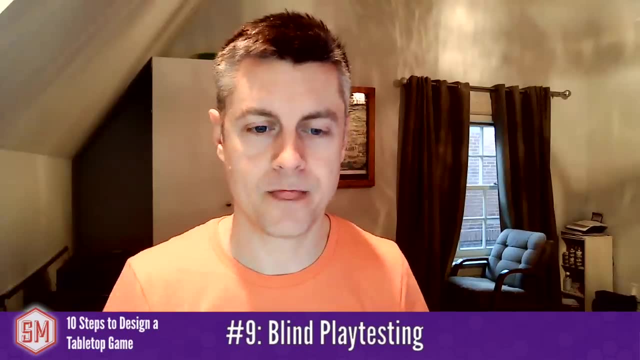 If you share it, you might find that other people are excited about it and they might be willing and eager to playtest it. I'm talking largely on social media, but you can also do this locally. But social media is a way to get blind playtesters from around the world. 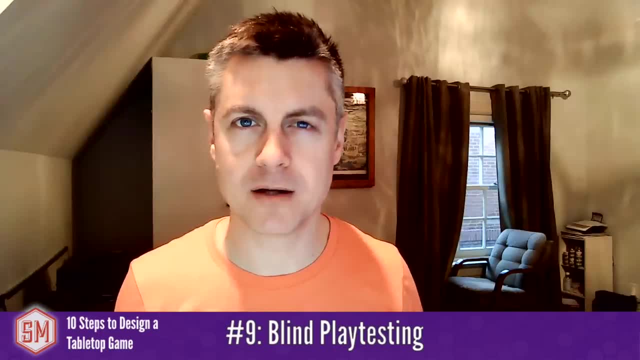 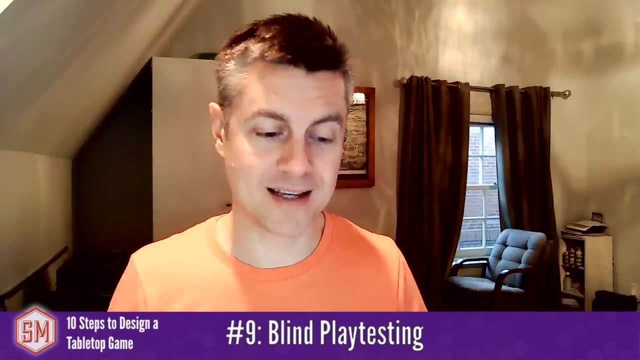 One thing that might- I don't know, I don't know- That might come to mind here is: should you be afraid of people stealing your game, stealing your idea? And no, Actually, the best thing you can do is put it out there and share it with people, because 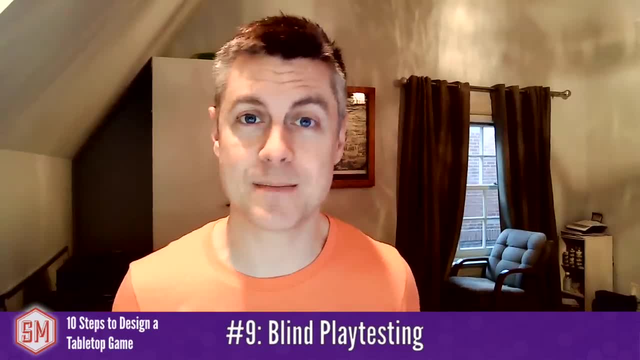 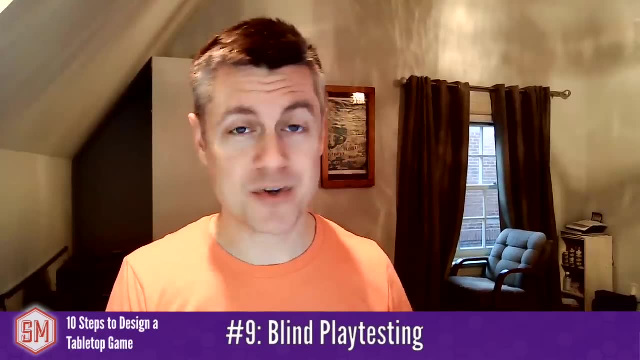 then people can always trace it back to you. If someone else does end up somehow stealing that idea- which is extremely rare in the industry, where they steal your exact concept- you can go back and say: actually, I was talking about this way before you did. 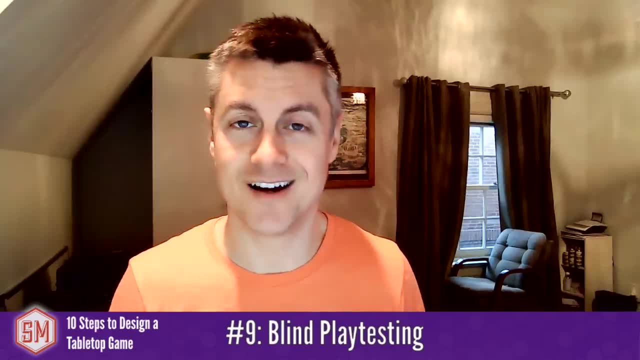 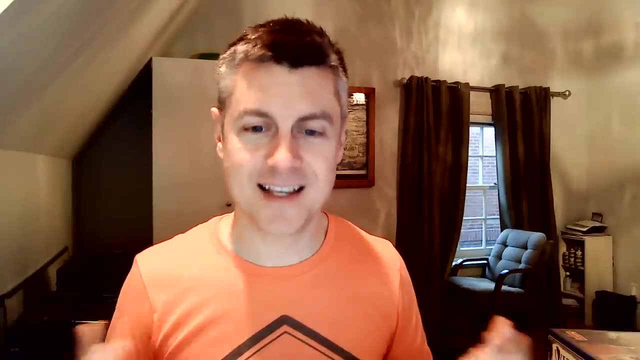 This idea originated with me. This game originated with me. You shouldn't be doing this. You shouldn't be publishing this game. That's blind playtesting. step nine, Finally, step 10, is: how do you know when it's finished? 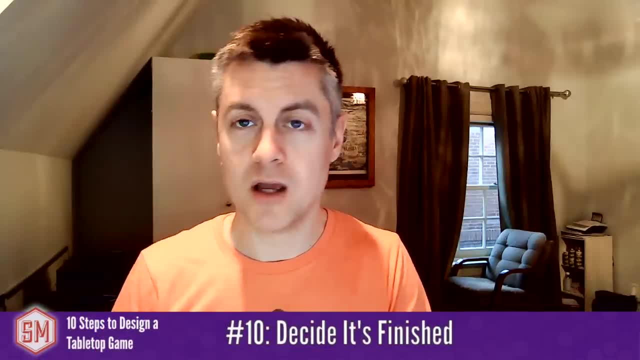 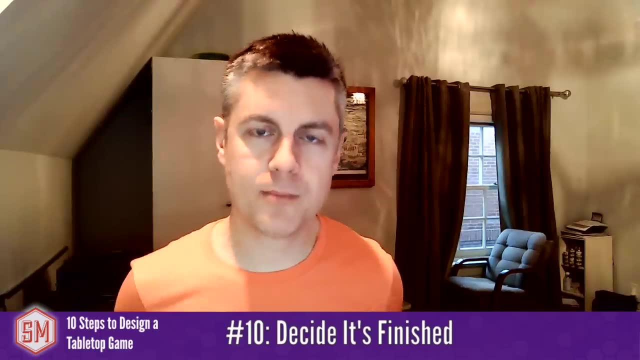 Step 10 is deciding: okay, this game is done, This is ready for me to self-publish or for me to submit to publishers. And this is a tough thing to know. When is the game actually finished For me? I usually put our games through between three and four waves of blind playtesting. 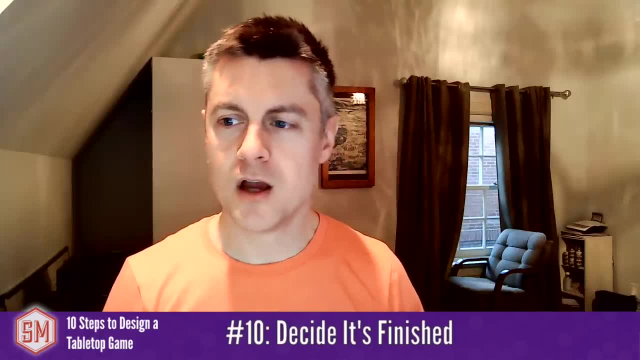 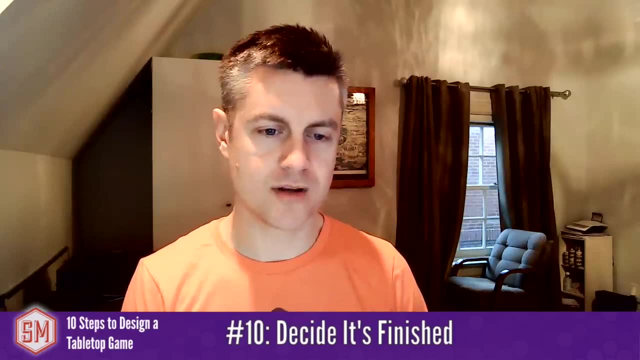 sometimes more, sometimes less, And usually by the third or fourth wave we're getting down to the really nitty-gritty. We're trying to get it as balanced as possible, trying to wrap up those rules and figure out all the final little rule questions. 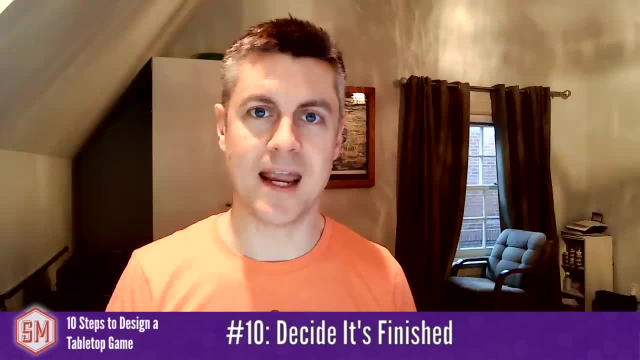 And I'm always asking playtesters to rate the games on a one to 10 scale. So as I see those ratings go up and up and up and I kind of see them plateau around eight or nine, then I know, okay, I think we're really we're getting very close to. 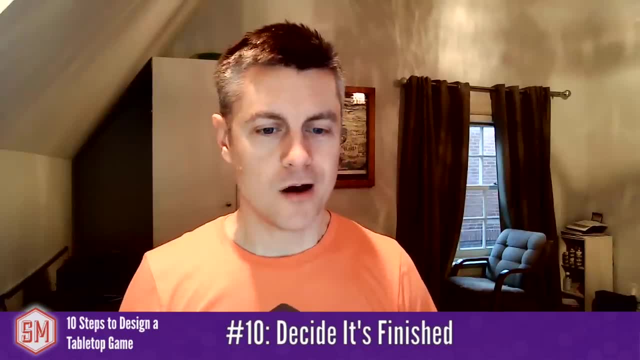 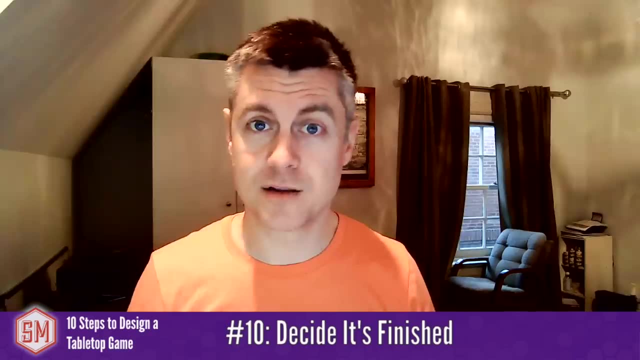 it. The game is very ready or very close to being ready. Also, part of it is instinct. It's just gut instinct. Oh, the game. I think the game. based on all this other information I had, based on my gut instinct, I think it is ready. 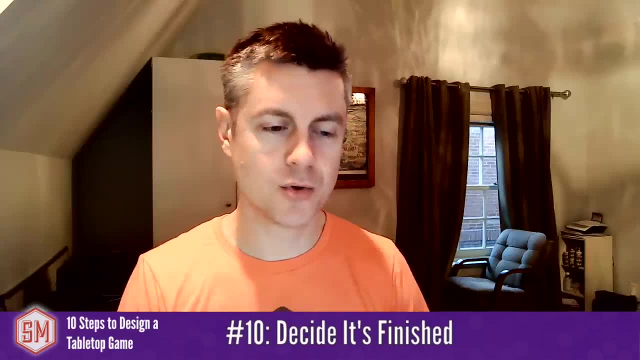 And the last is balance. All this blind playtesting is done for balance, So that you can look at someone, Some of the data that you're getting from blind playtesters, like how long did the game take to play? Who won the game?